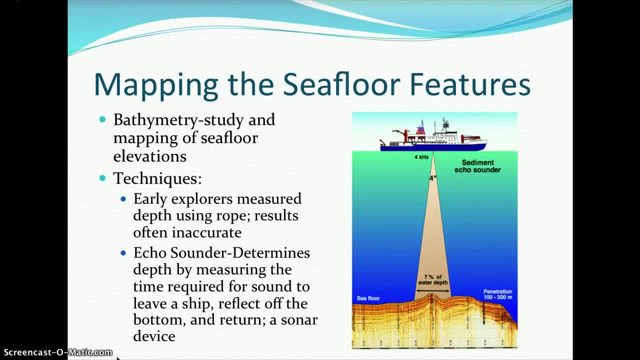 technology. scientists developed this thing called an echo sounder, And an echo sounder determines the depth by measuring the time required for a sound to leave a ship and reflect off the bottom and return back to the ship to where a sonar device was located. 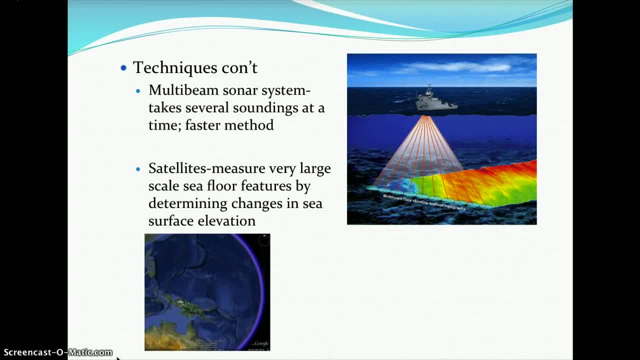 There's also a multi-beam sonar system and this takes several soundings, And when you talk about soundings, it's several measurements at the same time. This is a much quicker method for doing ocean bathymetry, because you could scan a seafloor and a seafloor and measure the depth of the ship. 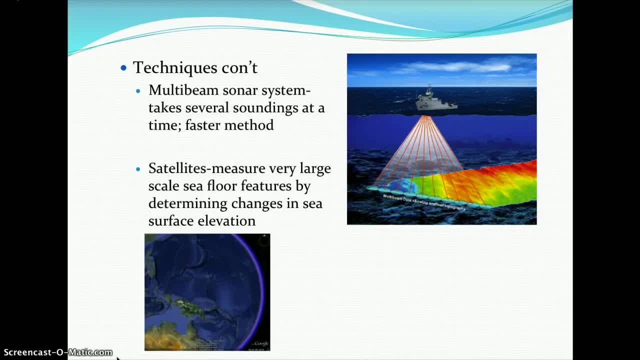 So you could measure the depth of a ship by measuring the depth of the ship and the depth of the seafloor. And even further advances in today's day and age. we can now use satellite imagery And satellites measure very large scale seafloor features by determining changes in sea surface elevation. 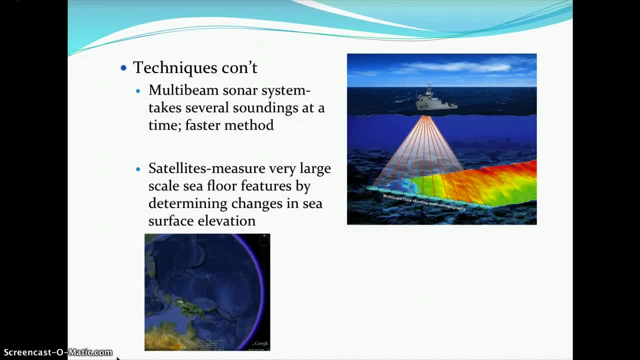 So, as you often know, that water is displaced when you put an object into it. so you can measure the surface elevation of seawater and try and get some type of idea of the type of seafloor features that are found at the bottom of the ocean. So here you can see. 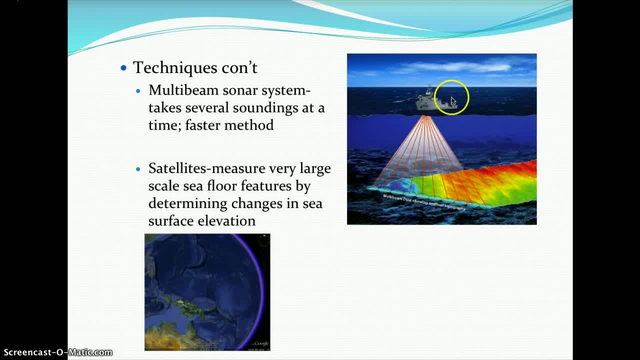 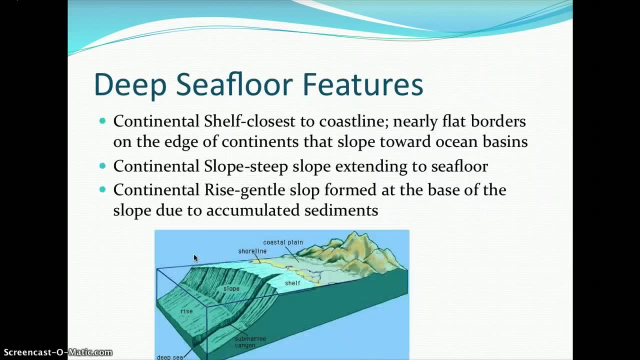 that multi-beam sonar system coming off of a research vessel there and over here. this would be a representative of what satellite imagery would look like when you're measuring bathymetry, and we will do an activity online related to ocean bathymetry. So what are some deep seafloor features You've all heard of at? 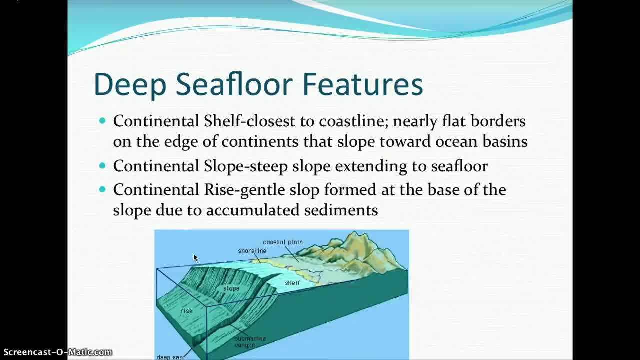 one point of the continental shelf, continental slope, continental rise, Whether you've studied this in your basic oceanography class, in earth and space science in middle school, or if you're watching a movie like a thousand leagues under the sea or some type of Discovery Channel you may have heard of. 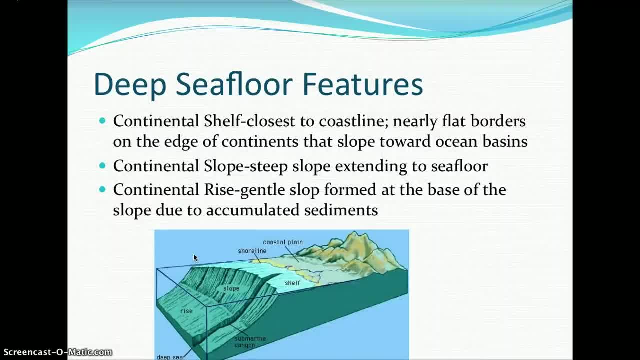 Discovery Channel program. you may have heard of the shelf of the slope of the rise. So these three basic features. the continental shelf is close to the coast line. It's nearly nearly flat borders on the edge of the continents that slope toward the ocean bases, basins. It is the continental shelf typically where, if you are 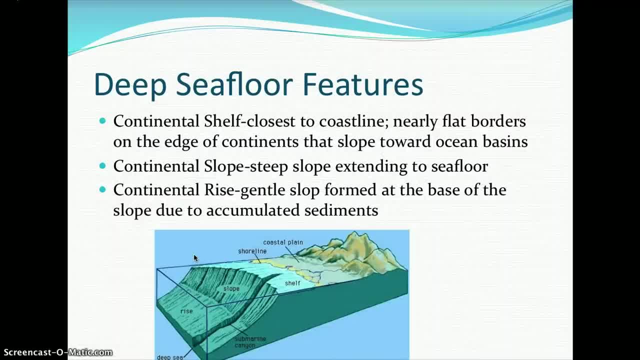 swimming in the ocean. you're swimming in this region of the seafloor. The continental slope is a steep slope that extends to this, extending to the bottom of the seafloor, and then you have the continental rise. The continental rise is a slope formed at the base of the slope of the continental slope due to 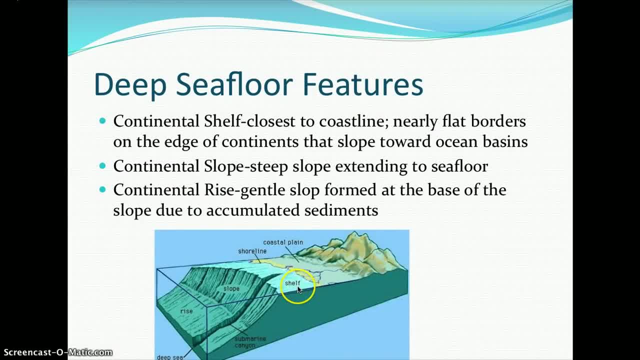 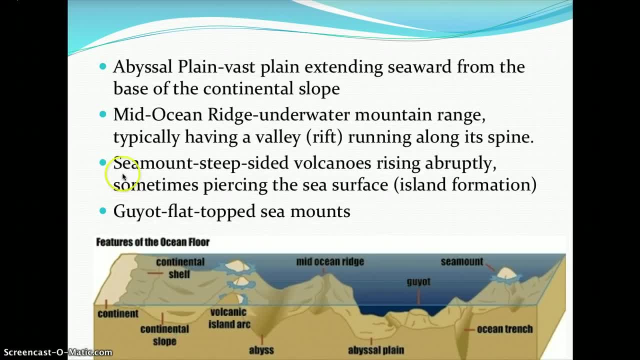 accumulated sediment. So here's your continental shelf, your continental slope and your continental rise: The abyssal plane. when you travel into the abyss, the abyssal plane is a vast plane extending seaward from the base of the continental slope. So here you have the, the continental shelf. 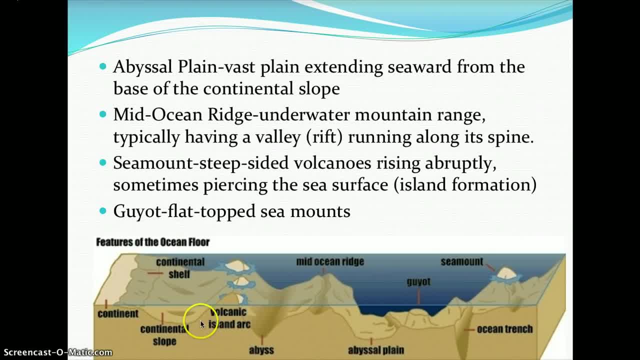 Continental slope, Continental rise would be that little area there, and down here would be the abyss. A mid-ocean ridge is an underwater mountain range, typically having a rift valley running along its spine. So here you have that mid-ocean ridge, That valley region. between the ridge will be the, the rift valley there. 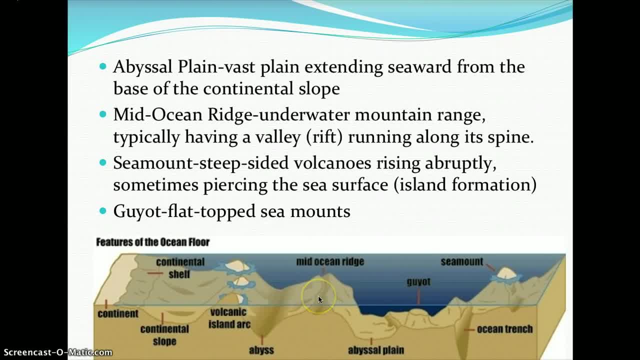 between the two peaks. This is what we saw when we looked at the mid-atlantic ridge. So the mid-atlantic ridge is that divergent plate boundary. We have new plate forming so you have a lot of volcanic activity there and you get. 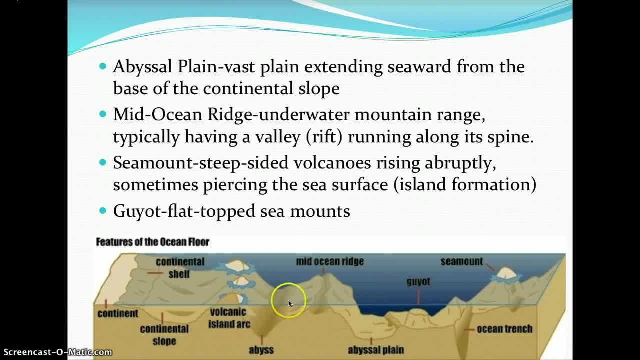 these ridge zones that would push the plates away from one another. A seamount is a steep-sided volcano rising abruptly, sometimes piercing the surface, creating island formation. So here you can see the seamount forming here. This here would be typical. a seamount will be typical with island. 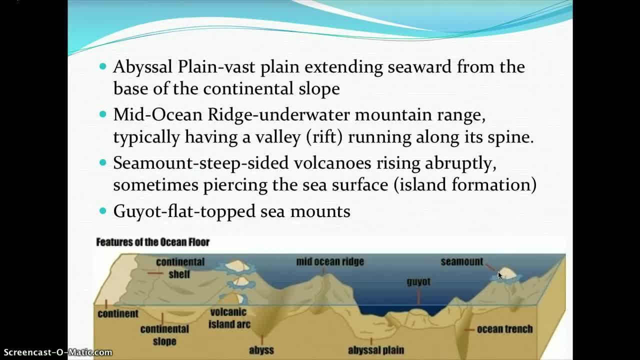 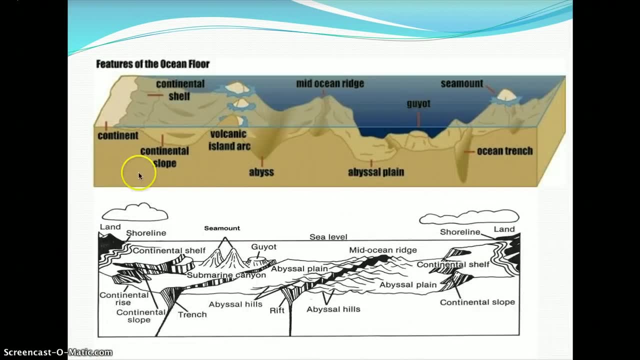 formation over hotspots. So the Hawaiian Islands are seamounts. And then you have a gaiope And a Gaiope is a flat top seamount. So due to erosion stuff you get that flat top there. So if we look here we see another diagram. so here we have the continental 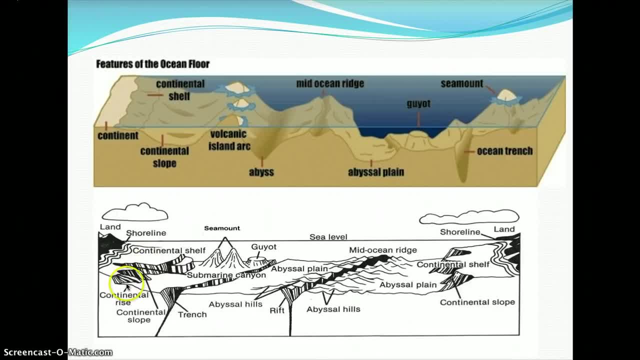 shelf. here's the continental slope, and then you have the continental rise here and now you have the trench, the abyssal plain. Here you have that ridge and rift valleys. So the ridge will be the mountain ranges, The The Rift Valley would be the valley between them. 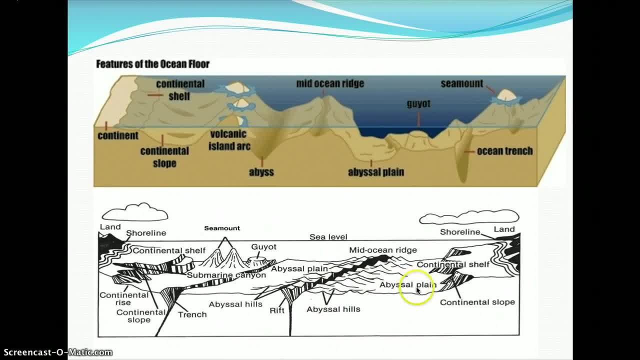 Here you have the Abyssal Plain again. Now we're coming over towards the other continent. Here you have the Continental Shelf, Continental Shelf- here Where's my arrow? Continental Rise, Continental Slope, Continental Shelf, Shoreline Land- A trench is a long, narrow depression of the seafloor. 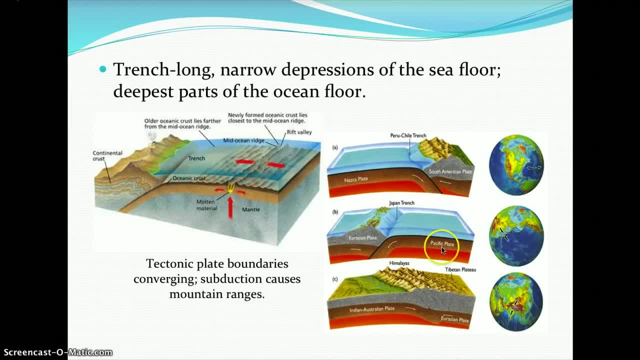 It's the deepest part of the ocean floor. Remember, this is occurring at subduction zones. so where you have plates one sliding beneath the other, you get trench formation, Tectonic plate boundaries. convergence of subduction causes mountain ranges. 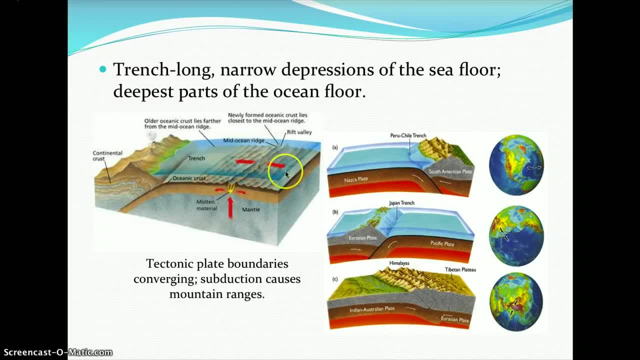 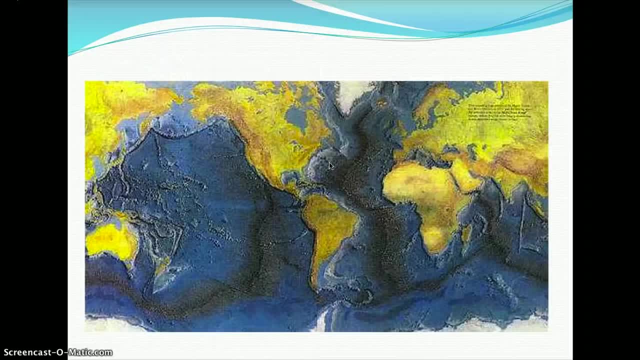 You may have heard of the Marianas Trench out in the Pacific Ocean and you did that in your one activity. You had to map that And then if we look so here we could see here is that Mid-Atlantic Ridge, here with the Rift Valleys. 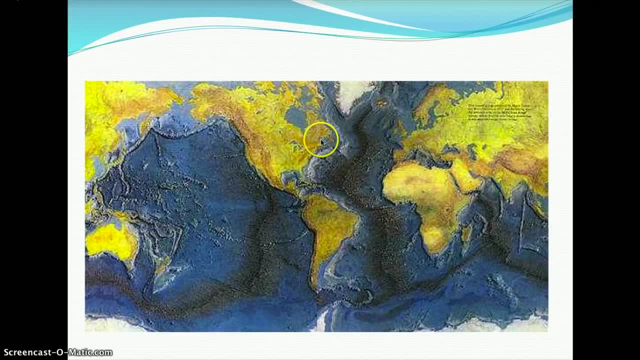 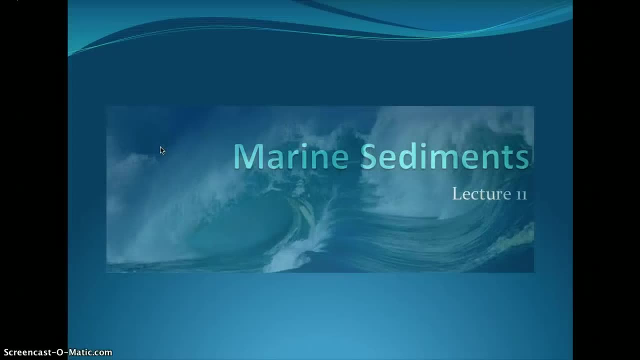 and then they're pushing towards the Africa and Eurasian Plate, and then over here towards the North American Plate and South American Plate, and then here is the East Pacific Rise. So you have the Pacific Rise there, or the Ring of Fire. Types of marine sediment. 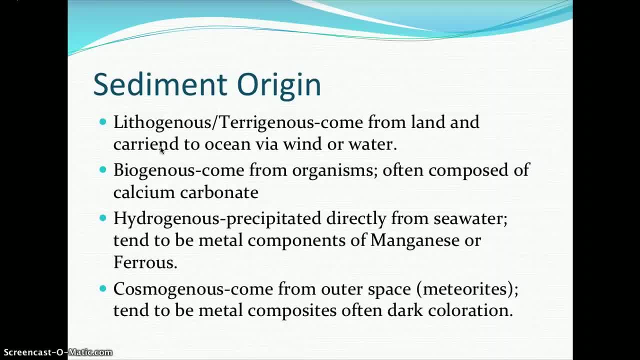 There are four different ways marine sediment can be found In the Old Testament. there's a lot of different ways marine sediment can be found. You have ocean or its origin. You have lithogenous or terrogenous sediment which comes from land and carried to the ocean via wind or water. 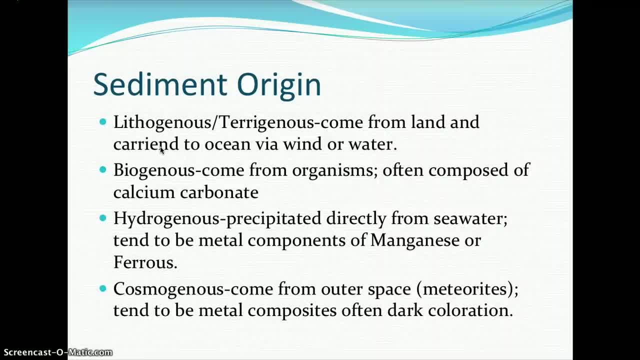 Biogenous sediment comes from organisms also composed of calcium carbonate. That would be some type of shell or hard casing that that organism was found in. You have hydrogenous sediment, which is precipitated directly from seawater and tends to be metal components of manganese or ferrous, which is iron. 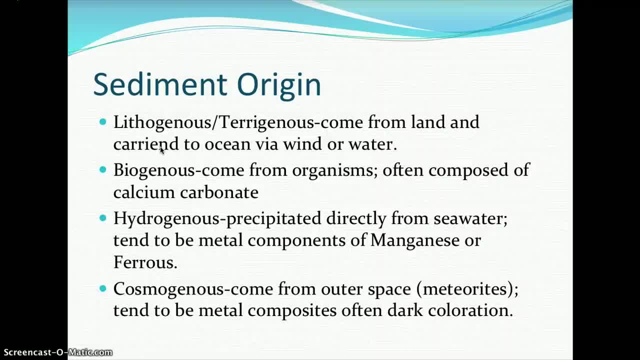 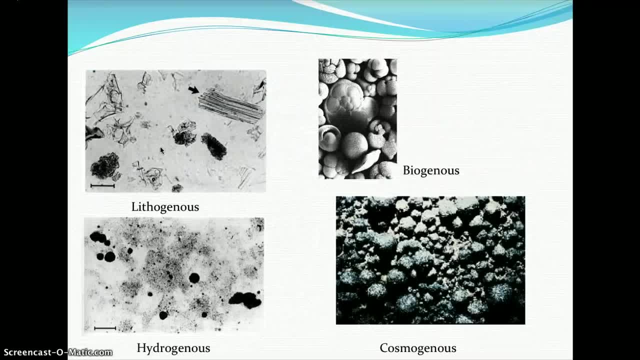 And then you have the ocean, And then you have cosmogonous sediment which comes from outer space, such as meteorites, and they tend to be metal composites, often darker in coloration. So here you can see what typical lithogenous sediments look like. 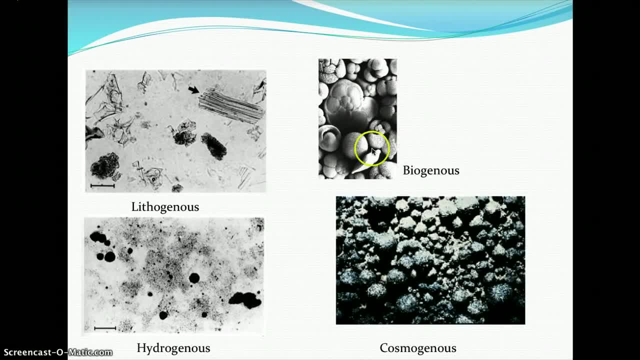 Biogonous sediments. this is pictures of foraminifera and we'll look at some of those in lab. Here is hydrogenous sediment which is precipitated out of seawater And here you can see that darker coloration of cosmogonous sediment. 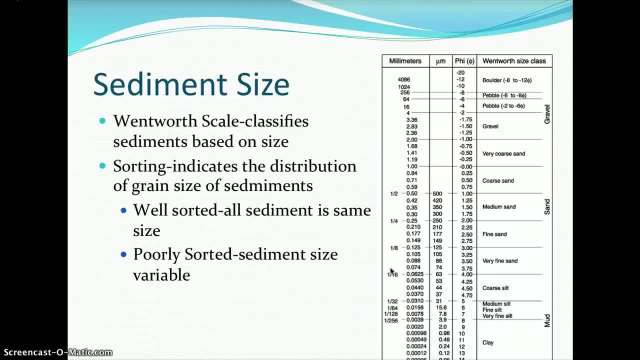 from meteorites. So when you go to the beach you know, depending on what coast you're on. if you're on the coast of New Jersey, you have that very fine particle sand, But as you travel north towards New England states. 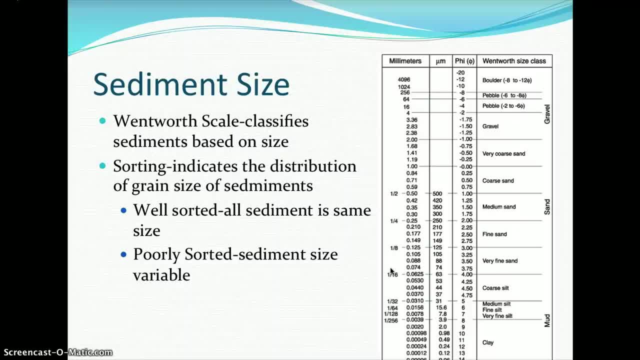 you don't have that very fine sand anymore, You start to have pebble and cobblestone beaches. So when you talk about the sediment size that can be found at the beach, you're going to use the Wentworth scale, And the Wentworth scale classifies sediment. 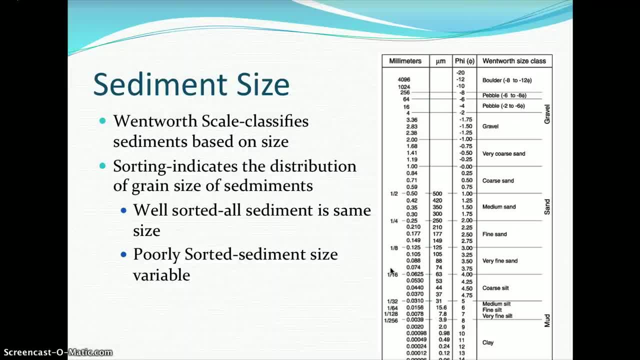 So when you talk about sediment size that can be found at the beach, you're going to use the Wentworth scale, And the Wentworth scale classifies sediment based on the size. Sorting indicates the distribution of grain size of the sediments, So you could use the Wentworth scale and a sorting technique. 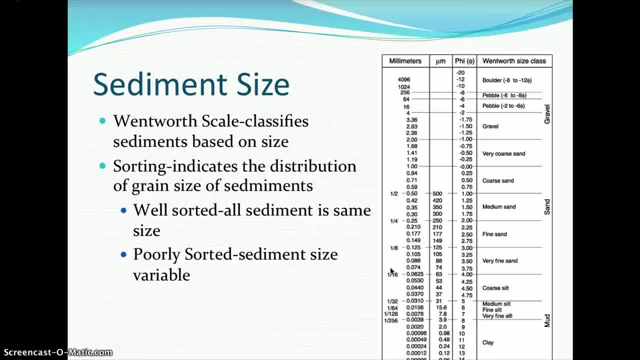 Some of us we did this in environmental science, where you put it into a sediment sorter and you shake it up and there's a little screen at each level and the particles will pass through. So a well-sorted beach is when all the sediment is the same size. 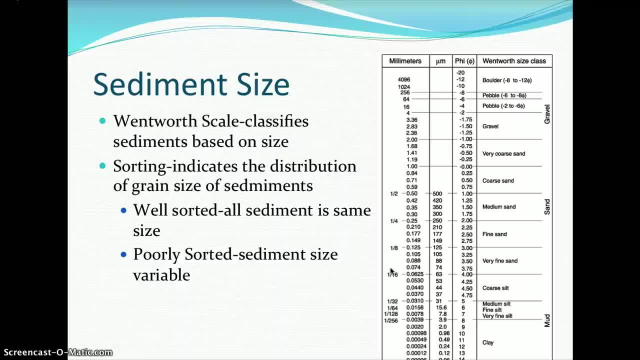 This would be very typical of the New Jersey coastline. where are those sandy beaches? Poorly sorted sediment beach would be up in the New England coast where you have rocks, pebbles, sand, So that would be poorly sorted. The sediment size is very variable. 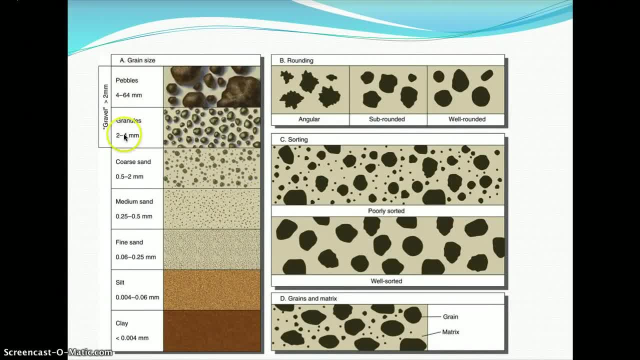 And here you can see So the grain size: pebbles, granules, coarse sand, medium sand, fine sand, silt and clay. This would be typical of grains, and matrix Here would be well-sorted, where the particles are all relatively the same. 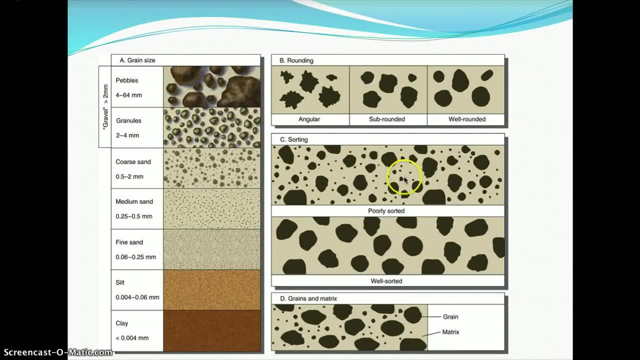 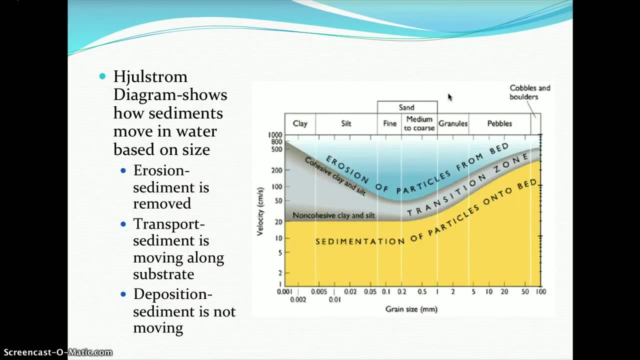 Here would be poorly sorted, where you have roughly different sizes, various sizes here, of sediments found in that sand. And then here you have a description of what that sediment looks like. Is it angular, sub-rounded, well-rounded? The Holmstrom diagram shows how sediments move in water based on their size. 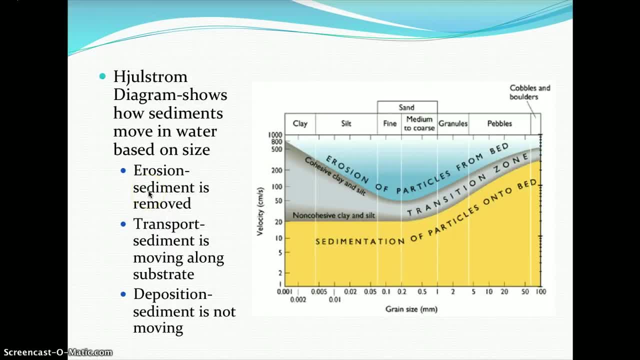 So basically we know that erosion is an erosion type process. Sediment is going to be removed And then you have the transport of that sediment. So sediment is going to move along a substrate or the bottom, in the bottom of the ocean floor or river, or being suspended somewhere. 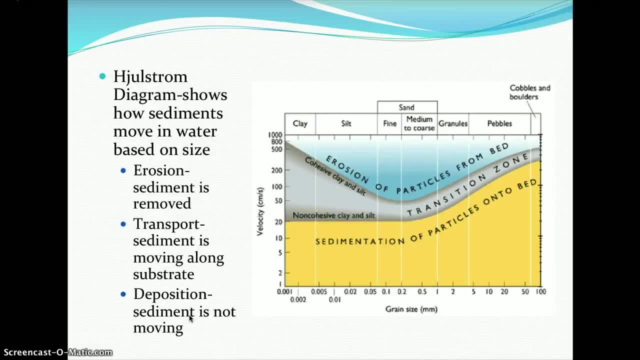 And then eventually you have deposition, where the sediment is deposited somewhere, So it's no longer moving, So erosion picks it up. Then you have that transport method And then eventually you have deposition, depending on the particle size. So here you can see the erosion of particles from the bed. 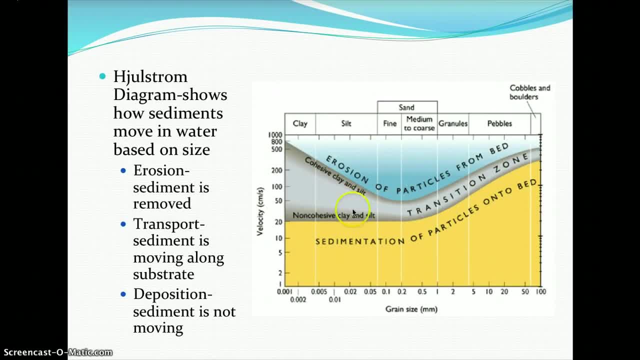 Here you can see that transition zone And then you have the non-cohesive clay and silt in that transition zone And then you have the sedimentation of particles into the bed. So you can see these three different areas here and the velocity of those particles in these zones in centimeters per second up the y-axis. 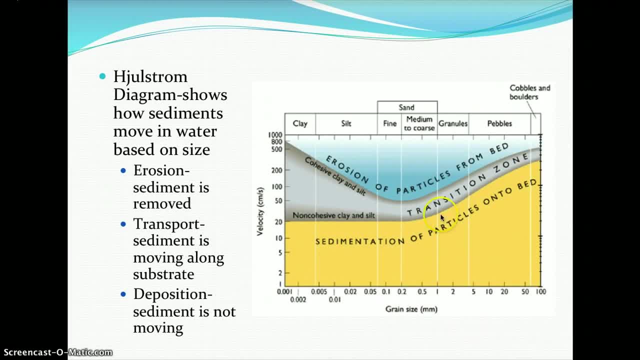 And then you can see the grain size in millimeters along the x-axis And up here you can see the various ranges of what those grains are. So down here In this zone you have clays In this zone here from 0.005 millimeters up to about a little more than 0.05 millimeters, you have the silt. 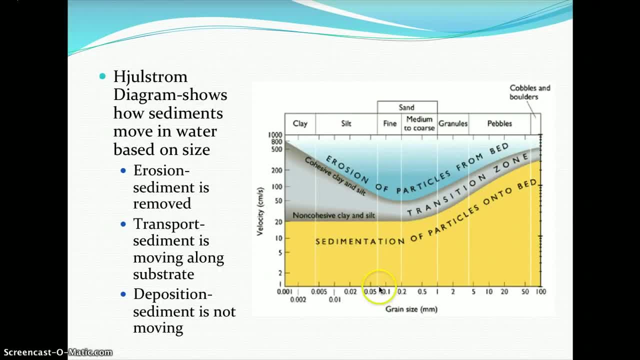 Then you have your fine and medium to coarse sand, which is a little bit above 0.05 and extends all the way up to 1 millimeter. So think about 1 millimeter and how big that is on a meter stick. And then, of course, you have pebbles. 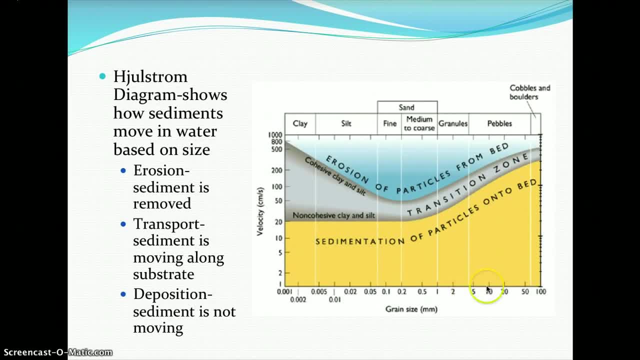 that range from a little less than 5 millimeters up to about 50 to 60 millimeters in size, And then much larger than that are the cobbles and boulders. So there you can see the Holstrom diagram and how it will relate to that Wentworth scale. 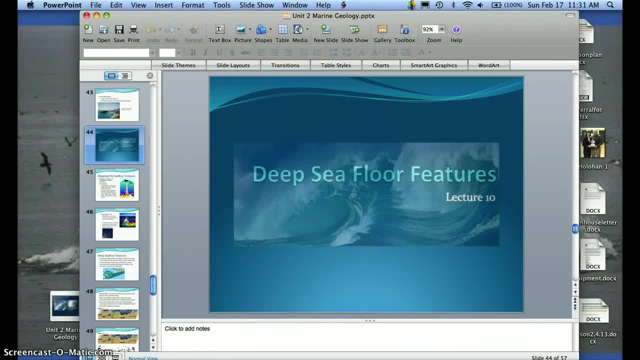 And that's all for geological oceanography. Everyone have a great day.